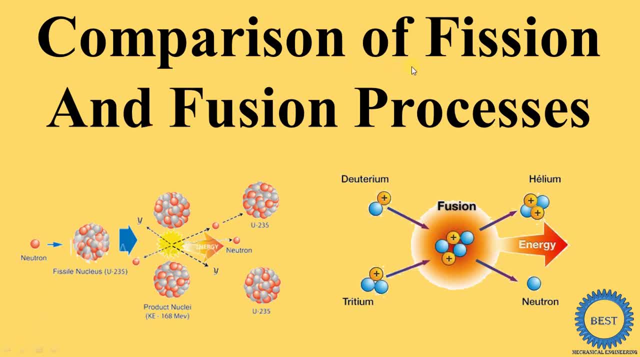 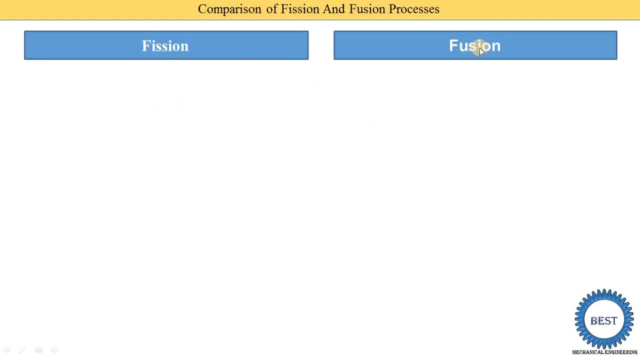 In this video I explain comparison of fission and fusion process. Left side we mention the point of fission process and on the right side we mention the point of fusion process. First point is a heavy nucleus split into two or more lighter nuclei means in a fission process the nucleus is divide means it is split in a two or more lighter nuclei. 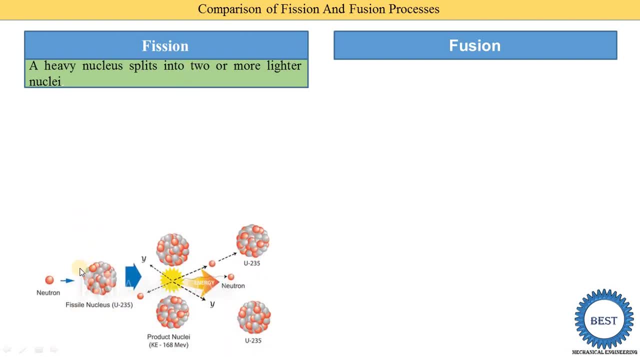 Means here nucleus is uranium 235 and on this uranium 235 we bombard the new tanks, Okay. So when we bombard the new tanks means uranium 235 is divide in a two parts, means it is split into a two or more lighter nuclei. So here you see, it is divide in a two parts, Okay, And this weight of the two part does not equal to the total weight of this uranium 235 means not equal to the weight of the nucleus. 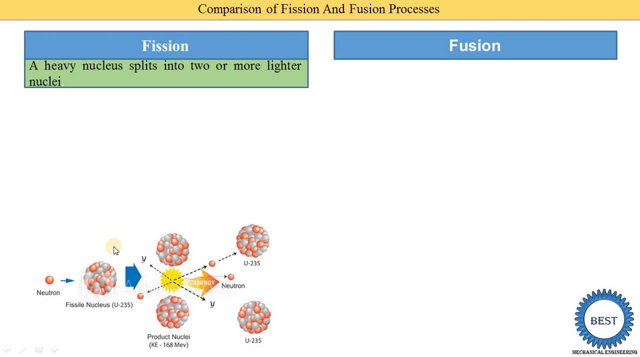 Okay, because when they are split, at that time some heat energy is released. so here you see, in between these symbols, the heat energy is released, or a heat energy is liberated- okay, that's why its mass is lower than the mass of the nucleus. okay means in a fusion process the nucleus is split into two. 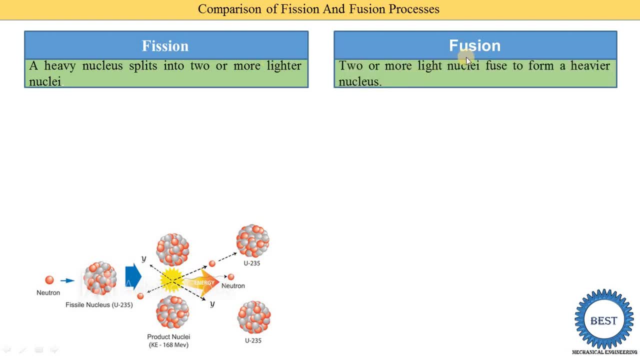 or more lighter nucleus. in a fusion process, two or more light nuclei fuse to form a heavier nucleus fuse means they are joint. now, here you see this image. okay, so this fusion process, this fusion process is carried out on these different hydrogen isotopes. okay, so here you see this, the deuterium. 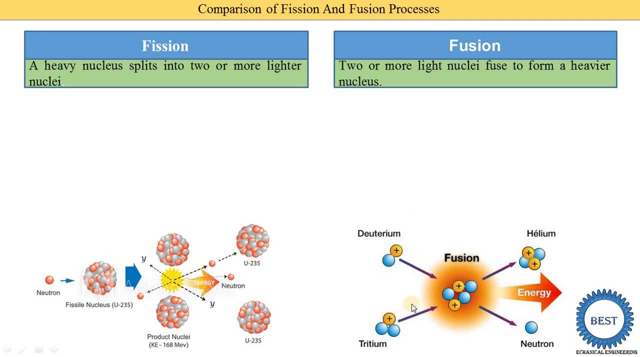 and tritums are the hydrogen isotopes. okay, so, here you see, these are the deuterium and tritums and isotopes and they are fused. fused means they are joined. so here you see, these are the here the two atoms and here the three atoms, and they are joints, and when they are joints, they release the. 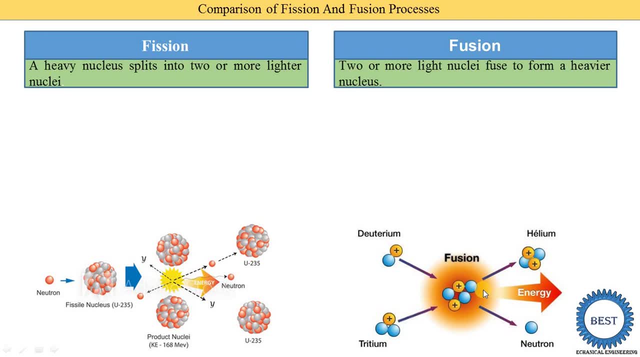 heat energy, okay, and when we need to do the fuse process means nucleus is fused, means they are joined. for this joining process we are required a very higher temperatures, okay, and after these reactions they are provide the heliums and the neutrons. you second point: fusion reaction does not normally occur in a nature, okay. so in this nature, in this. 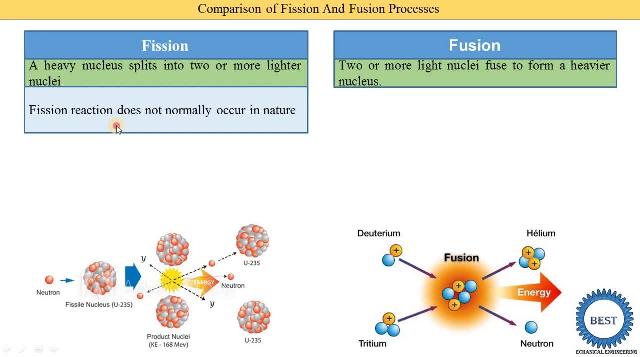 wall, that is a fusion process, is not naturally available. but fusion process are naturally available. energy liberated by the sun and the star is due to nuclear fusion. okay, so you know that the sun is emits the radiations. okay, so sun temperatures are the very high that is the gray esa temperature will cause more radiation. so if there is different product, 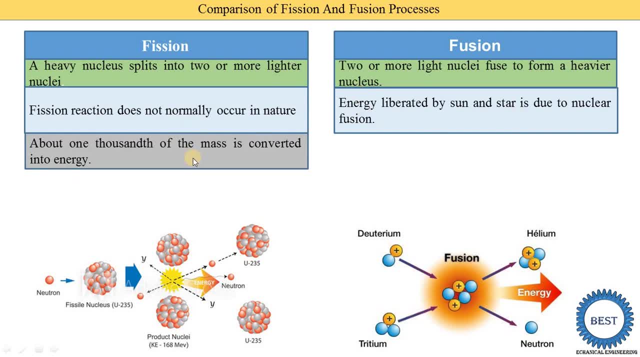 pressures. this temperature is high due to of the fusion reactions. so, in particular, this temperature is high due to of the fusion reactions. third point: about 1000 of the mass is converted into energy and in a fusion it is possible to have for thousands of massência converted into energy. 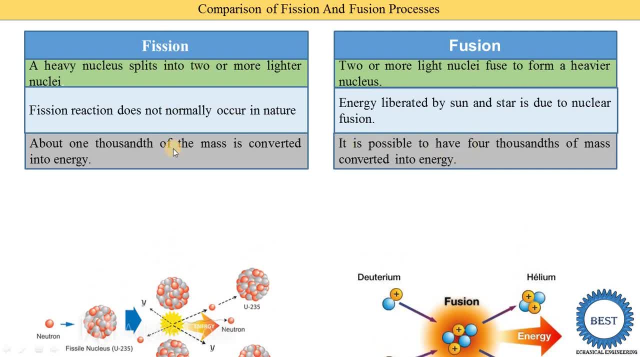 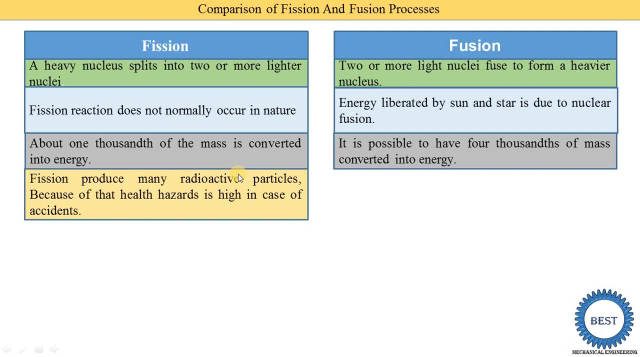 means during the fusion reaction more energy is produced compared to the recent process. Fourth point: fission produce many radioactive particles and due to many radioactive particles the health hazard is high in a case of accident In a fusion process. few radioactive particles are produced in a fusion reactions and due to that laser radioactive material. 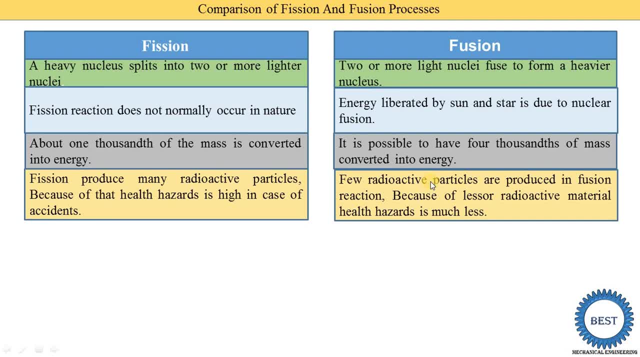 that means the health hazard is much less. The process is possible at the room temperature means fission process is done at the room temperatures, but the fusion process they are not possible at the room temperatures. for that we are required very high temperatures, because here the joining is carried out of the light nucleus. so joining process is required a very 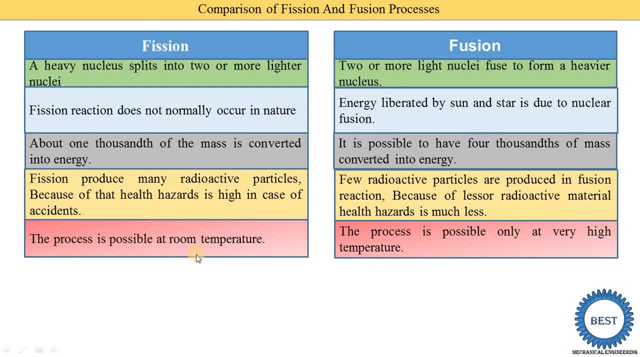 high temperatures and here the splitting process are there, so they are occurring at the room temperatures. This process give rise to chain reactions means the chain reaction is increased continuously and in a fusion process does not give rise in a chain reaction means they are not continuously rise For a fission. 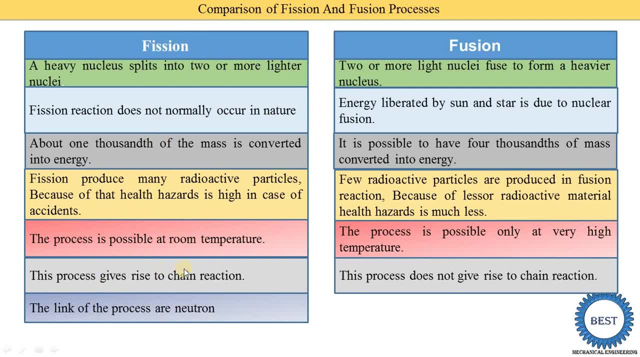 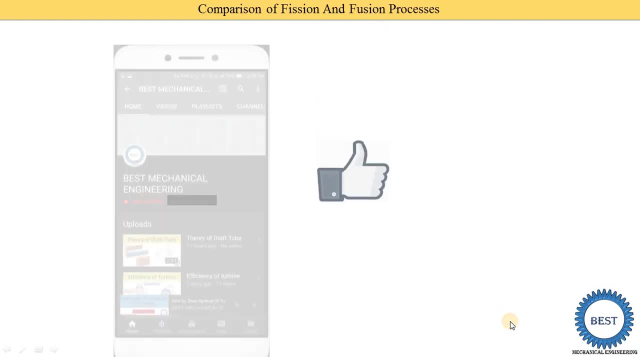 the link of the process are the Newton means this process is carried out due to the Newton's and the fusion process are carried out due to this. protons, or they are link of the process, are protons. Now, before moving ahead, I request to like the video and subscribe my channel for watching.